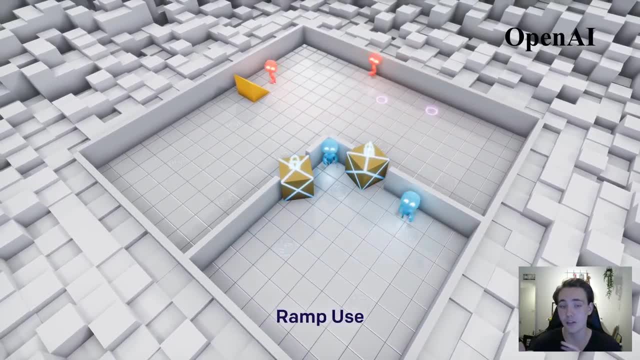 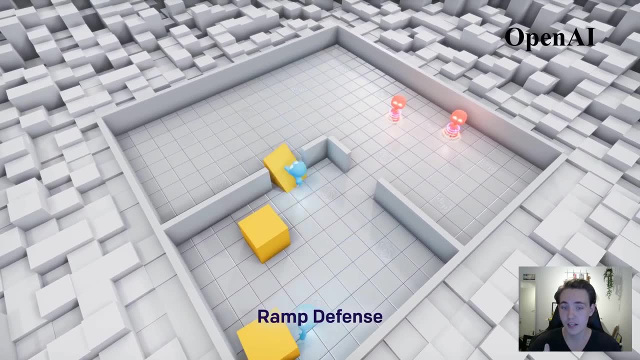 those boxes here and just um, keep hiding and learning by using reinforcement learning, and then the great agents also learns over time. so they have this ramp that they can play around with and try to use that ram to to like try to find, or like get over the walls here to find. 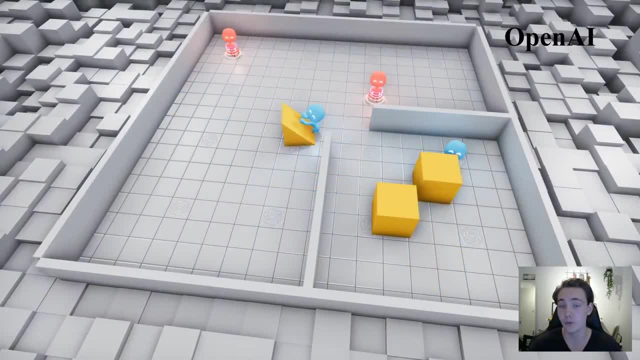 the blue agents. so in this case here we just saw that the blue agents there they're not. they've now learned to take to take the ramp here away from the red um seekers. so they can't find the blue ones because they they've shown that they have already blocked the entrance. but 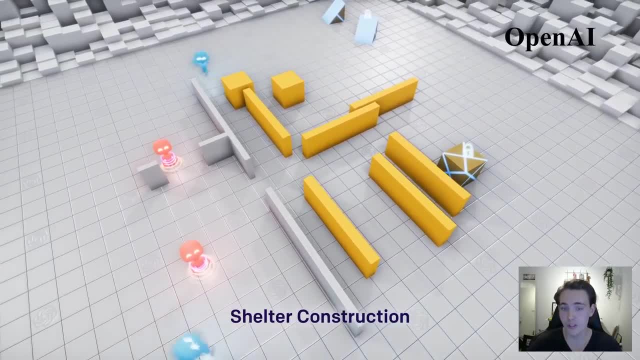 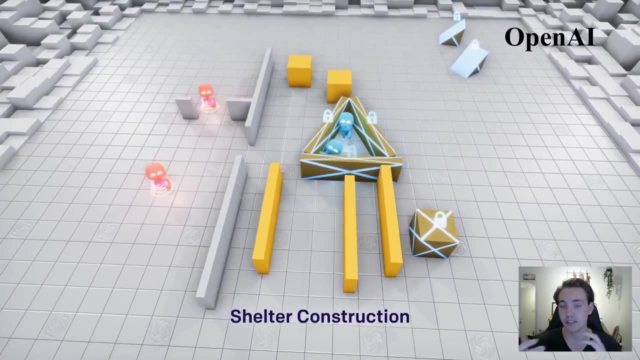 they could still, um, get into them by by using this ramp, and and then find them. and then they just learn over time that if they remove this ramp as well and block the entrances, then they, they can just like hide away from the red seekers, in this case. and here they're like making a. 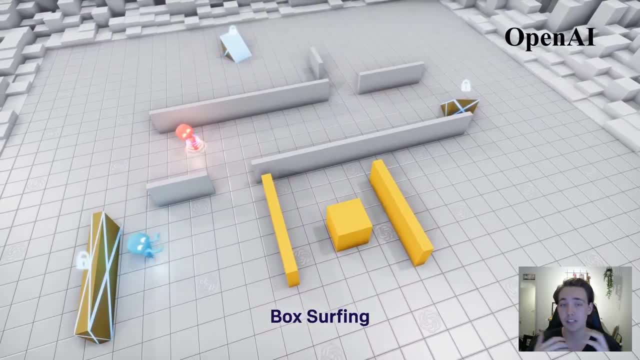 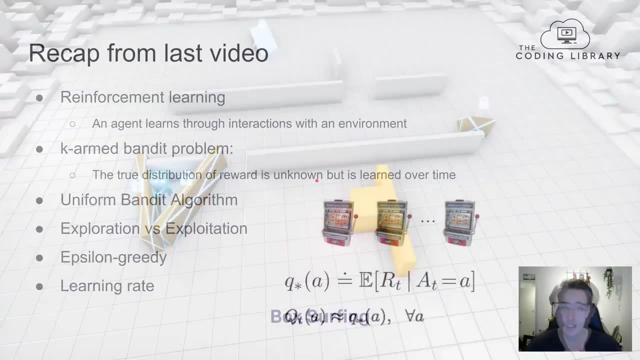 triangle and then over time when new objects are placed like they just keep on learning by exploring the environment and then just learning how to hide from from the red agents here. so first of all we're going to recap from the last video what we talked about in the last video, where we have 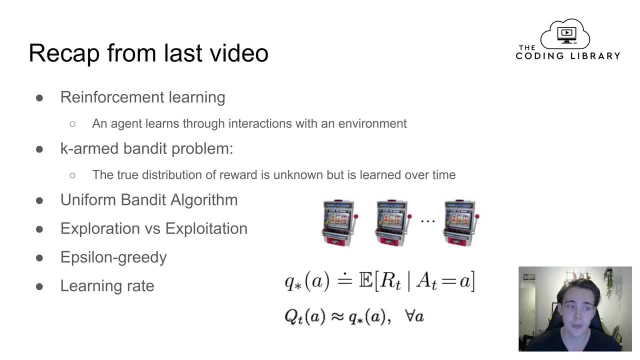 where we had a short introduction to reinforcement learning. so in the last video we learned that reinforcement learning, um, is where we have an agent that learns, that learns through interacting with the environment that is placed in, and then we talked about this example here with the k-arm. 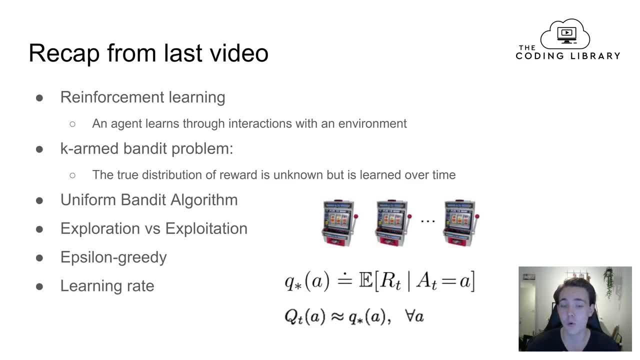 bandit problem where, like the true distributions of the rewards were unknown for um, for a lot of, like the slot machines, but it was learned over time by the agent by by using this exploration and exploitation which we talked about. so the agent was pulling the arm and and exploiting what 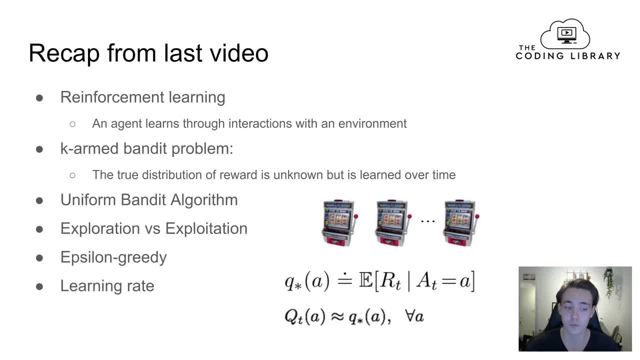 it already knew, and then at some epsilon greedy or, if we use this epsilon greedy algorithm, and then at some times some, at some point it was out exploring the other arms and trying to um find the distributions for the other arms as well. so in the end, when we were exploiting the environment, 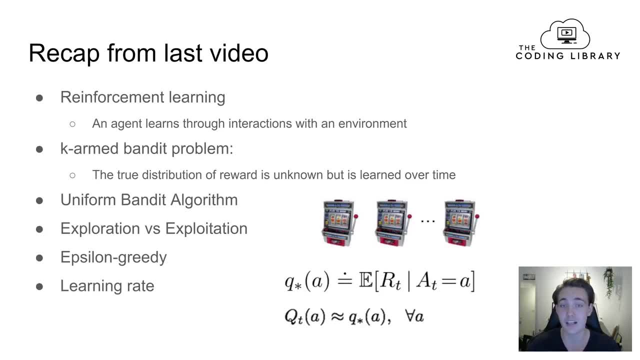 we were able to get the maximum reward. we also talked about like this learning rate, like how fast our agent has to, like uh needed to learn, and if we took two big steps or like two small steps, we will just hit it into a local or like a local minimum. and when we're using reinforcement, 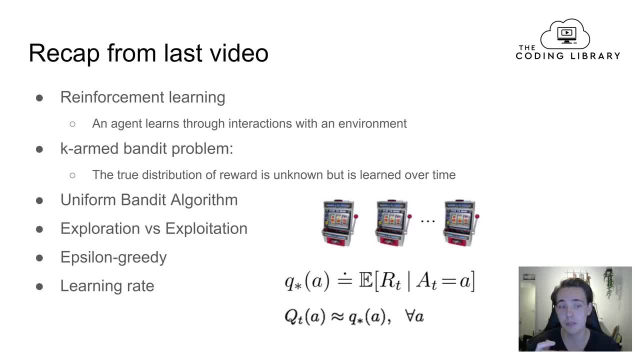 learning. we always like, want to to get the maximum reward and hit a global minimum and not a local minimum. so we talked about, like how we should determine the learning rate and and some other different kind of stuff, and saw an example of how we could use them in in. 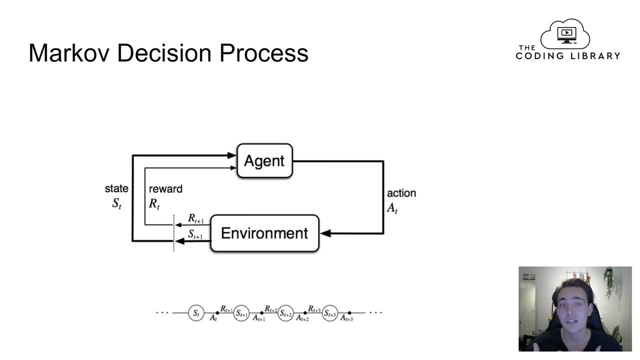 field example. so now we're going to talk about market decision processes and what it is and how we can use it in reinforcement learning. so first of all, we have this example here where we have a state for um, for the environment, and then that state is giving to the agent for some time. step 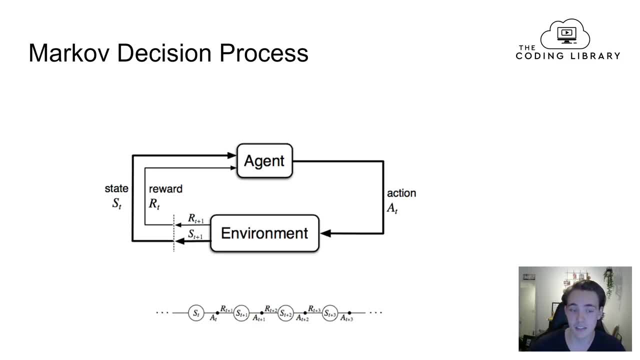 and also reward, if it was given a reward for some action taking. so from a given state the agent takes an action, at times that t? um in the environment and then from the environment, the environment like outputs a new state to time step a t plus one, and then for the action 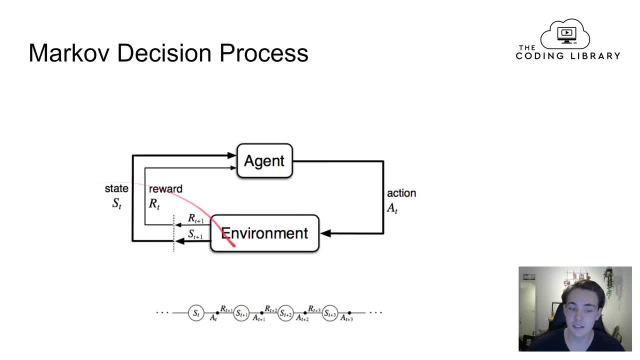 taking in the environment from from a given state t here. then it also gets a reward for the for the time time step plus one, and then the reward and new state here will be fed to the agent and then the agent can can take another action um from that reward and the state it was given from the. 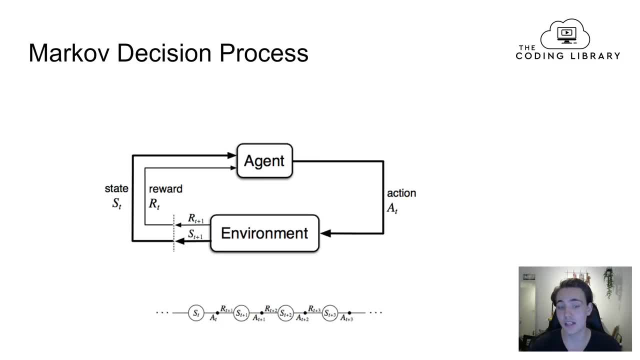 environment and then this process just keeps continuing until, like, our agents learn from the environment and stuff like that. so down here is just like, it's just like um, how to, how to like the timeline works. so first we're given a state here and then we take an action and from that action in the state, 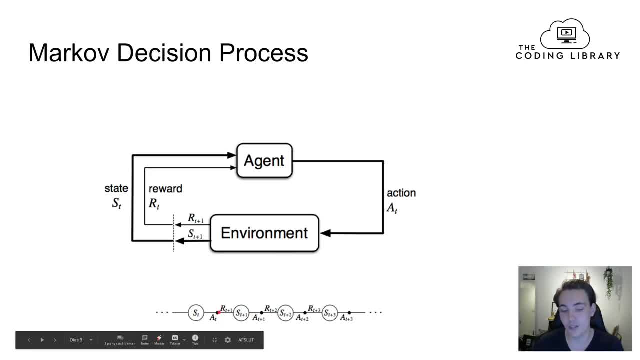 we, we get a reward here, and then we we're returned with a new state at an at the next time step, and then we just keep continuing this process again here, where, from the next state we're in, we take a new action and we get a reward from that action, and we do the same again for the next time step. 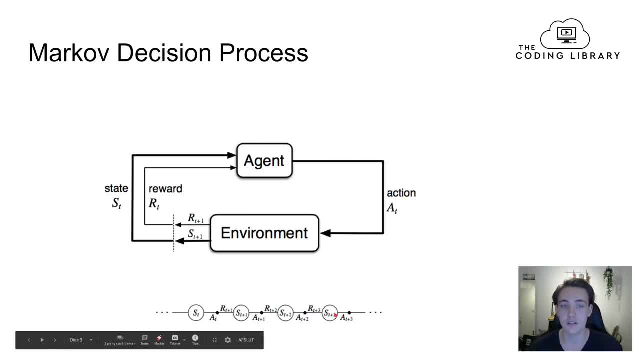 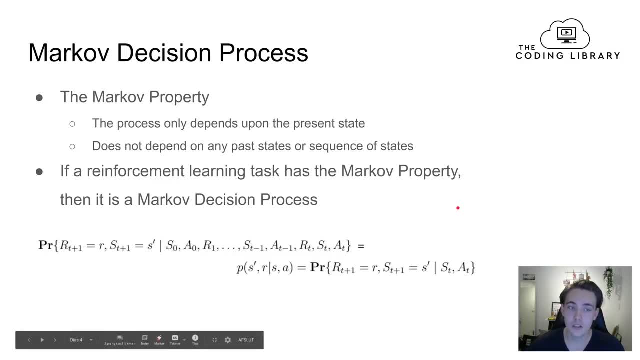 two here and three and so on. so like this is like how the, the, the process works in in reinforcement, learning, when we're talking about markup, decision processes, so when we're talking about markers, this process, we have this market properties. so our process, or like our application and reinforcement and learning and process, needs to have this market property. 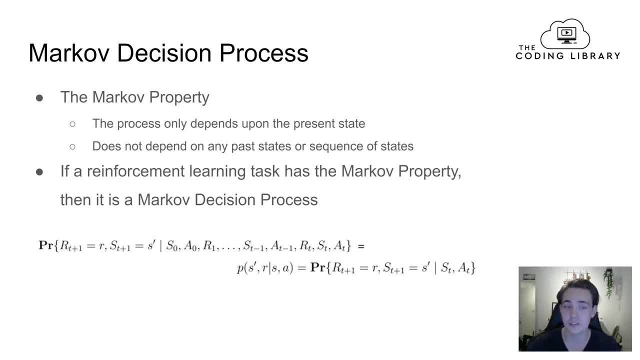 and the process only and we it has market profits, property, if the process only depends upon the present state, so the state we're giving right now is the only only thing that matters when we, when we're talking about, like, which action we should take and stuff like that, so it doesn't depend on. 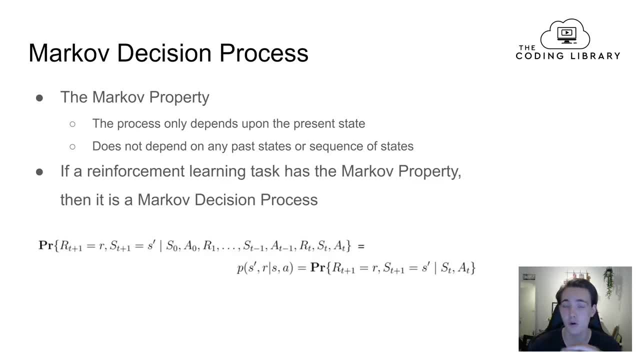 any any past dates or sequence of the previous days that we've already been in. so when we're talking about the market property, we don't care about the past stage. we only care about what state we're in now, and then we take the best action for the state we're in now and 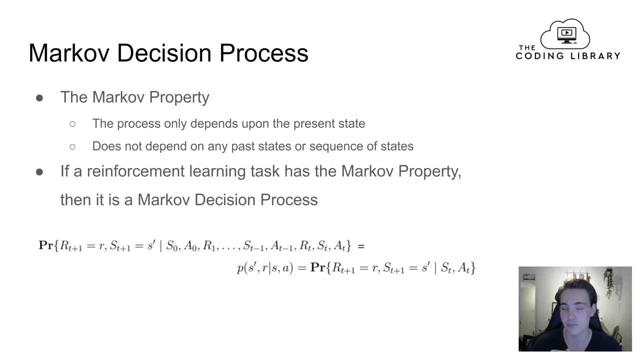 then we can say that our, our process has a markup property, and then we can use um, the, then we can use the methods and we're going over in this video as well. so if a reinforcement learning task has the market property, then it is a markup decision process. 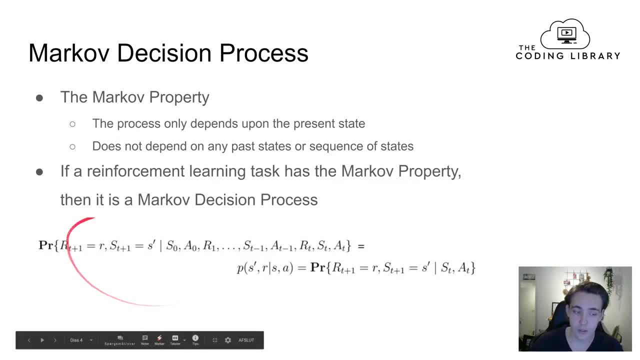 your, and then we just continue that. and then we have like this mark of decision process down here where we have like some probability of the next state and the reward for the next state given as state and an action that we take in this time step here. so this is like just like the mathematical, like 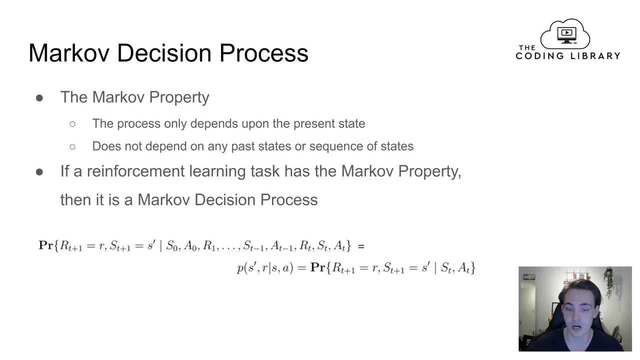 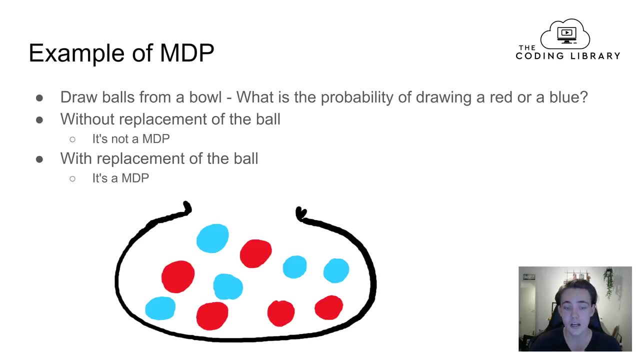 formulation like and for, like the mark of decision process that we're going to use as well. so if we're going to like have an example here of the mark of decision processes, we have just like a very easy example here, like, or a simple example where we draw. 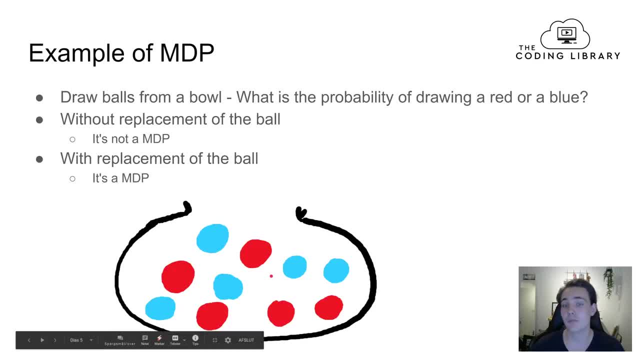 the balls here from a bowl and we can then say, like, what is the probability of throwing a red ball or a blue ball? and in this case here there are five of each, so the probability would be 50% of throwing a red ball or a 50% for the probability of throwing a blue ball. 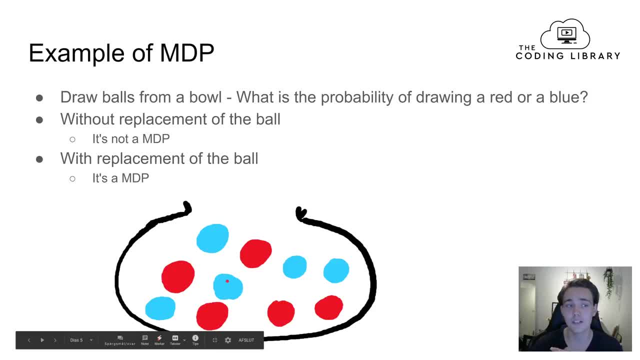 so if we want to like determine if this process here is a mark of decision process and if we want to like determine if this process here is a mark of decision process and if we want to it has market property, then it is not a mark of decision process. if we if, if we like, if it's. 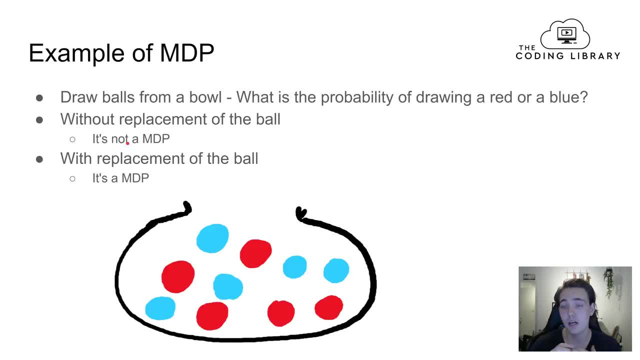 out with, without replacement of the ball. so if we take the ball out here of this um, of this bowl here after we have drawn it, then it won't be a mark of decision process anymore, because then then we we need to like the next action we takes and the next action we would take like with which? 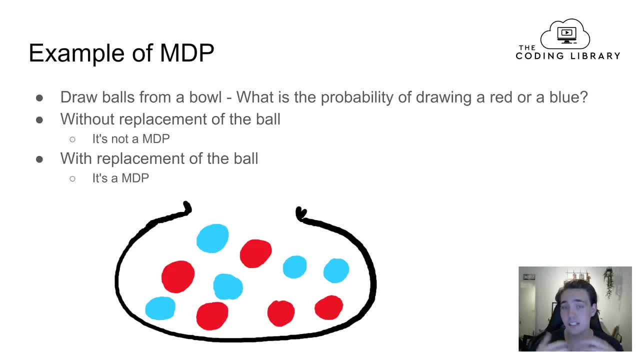 is throwing a ball. it will then like. it will then depend on previous state, because now we have removed one of the colors from from the bowl and it will not be a 50-50% probability of throwing a red or a blue ball. so if we had replacement in this example here it would be a mark decision process because 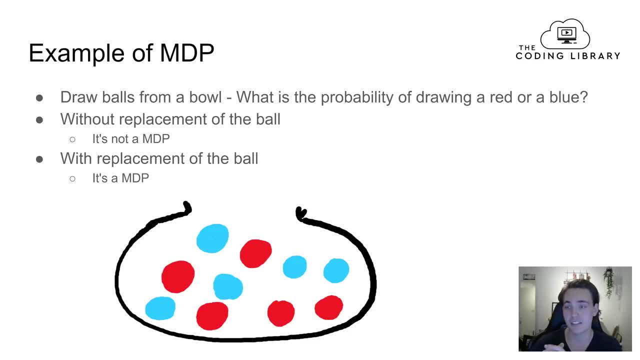 then it doesn't matter for any given time step like which action we're taking. we will still have 50-50% probability of throwing a red ball or a 50% probability probability of throwing a blue ball. so this is just a simple example of like how we can set up a process and and determine if it's a mark. 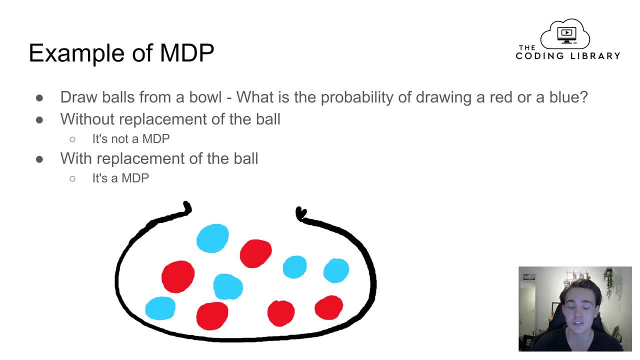 of decision process or not, because if it's a marker decision process and our action- taking like or the action we're going to take- only depends on the present state and not the previous, not the previous or past dates or or sequence of states before that, so we can also talk about like. 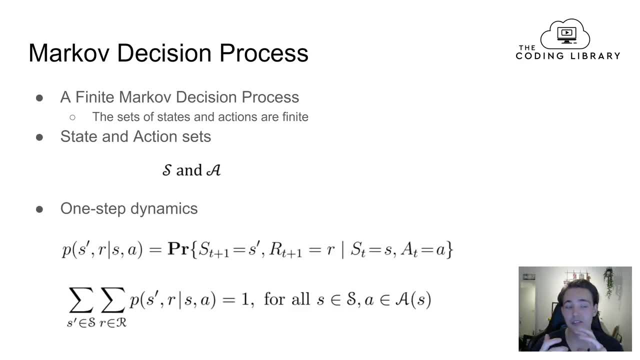 finite marker decision processes, which is where we have this finite market and market decision process. we have a set of states and and actions and then those sets are finite. so we have like a finite and a finite set of states and actions and then we have this, like this mathematical expression, like s and a, which is the set of the. 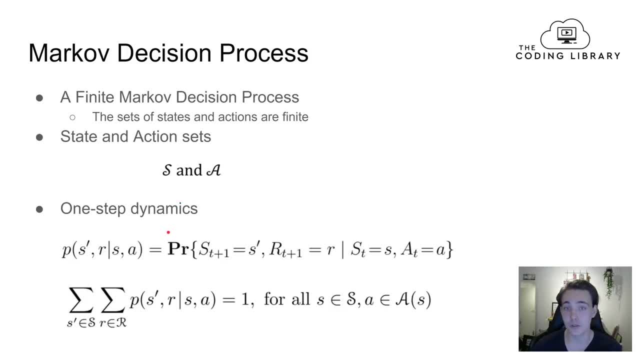 states and the actions, and then we can set up this one step dynamics which we're going to use in in and later in the on the next slides, where again we have this a probability here for for like, the next state and the reward, and then, given we have in the state and we take 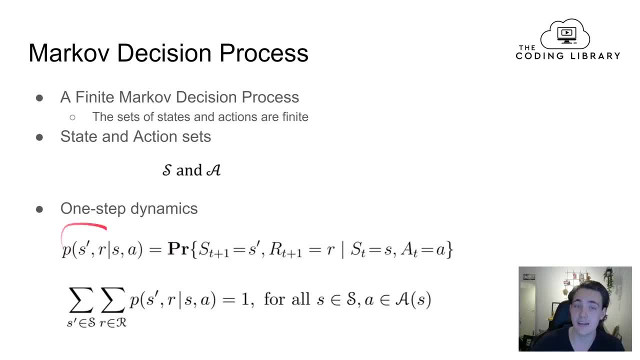 an action like what is the probability often, of the next state and reward given, as the state we're in now and the action we take, and then we can set up this one step dynamics which we're going to use um as well, and then we we end up with with some math here which is two, uh, two summations of of. 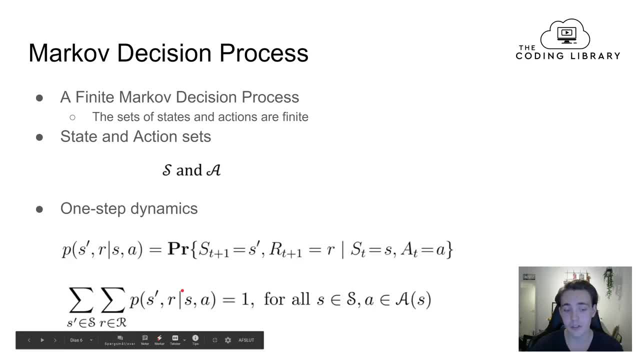 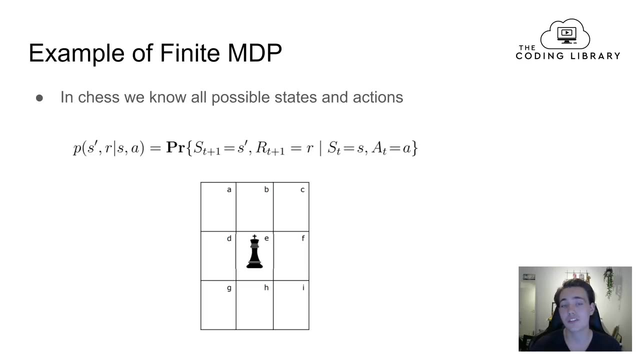 these probabilities here. they need to be one, uh, because the probabilities should always be like 100 percent. um, for all this, this sets in our, or like all the states, in our state set and all the action set given given a state. so an example of a finite mark of decision process is this check. 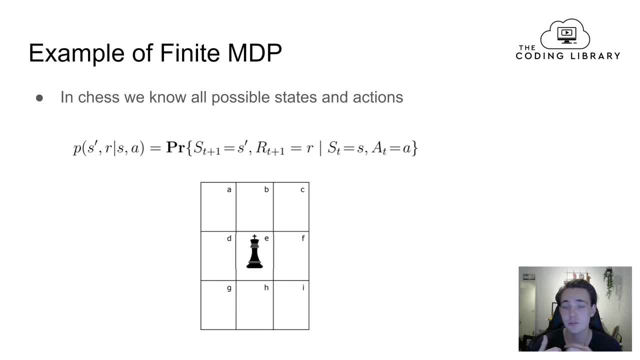 report here where, when we play chess, we know all the possible states and actions. so we have a finite um set of states and actions, because if we have this king example down here on the checkerboard, then we know all the states and all the actions, um, in this case here, and it's all. it also has Mark. 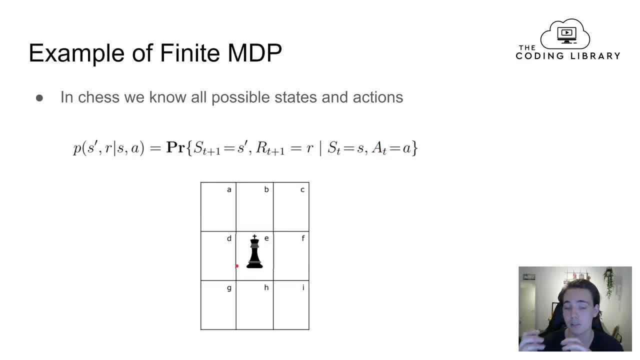 of decision property, because we only, it only depends on this date. it is in now and we don't really care like about, uh, the present state it has been in. so right now the king is in this state, here, is in the middle, and it can either like go in the direction, diagonal direction, or it could go to the left and right and 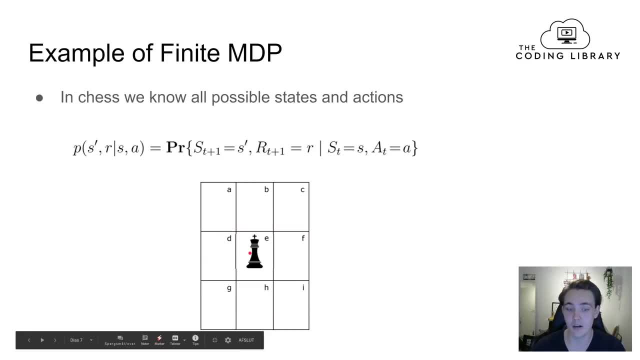 up. so these are the possible actions that this agent can take now and the states here are like. the possible is the checkerboard here. it is the state where it can go in in these directions here and which is the actions that you can take. so in this case, here we have a finite number like, or a. 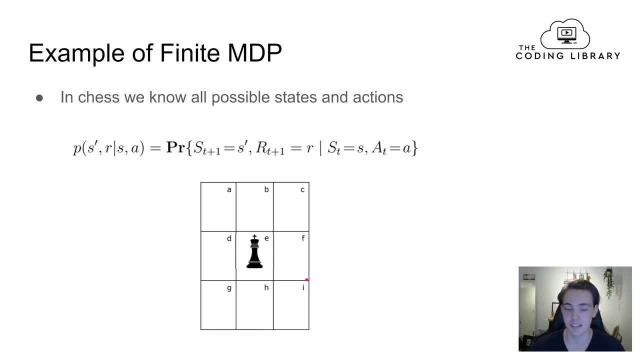 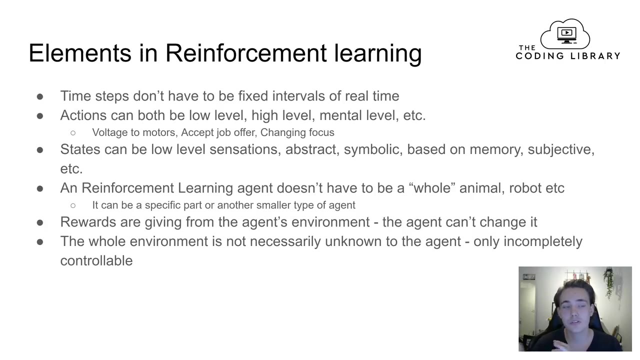 finite set of states and action that it can take in this example here, and this is like why, um, it is easy, or like kind of simple, to use reinforcement learning in in, for example, uh, chess, because we have a, a finite marker of decision process. so I also wanted to like to to tell you guys about, like, the elements. 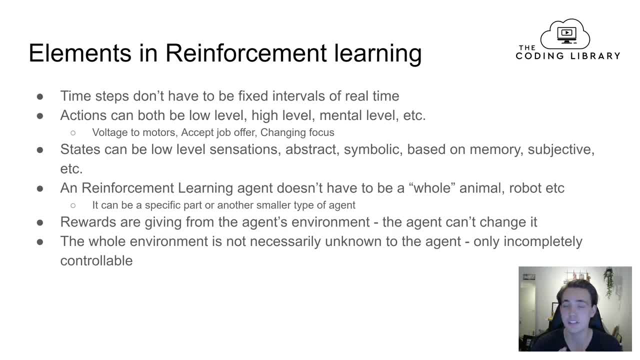 in reinforcement learning, like the different kind of elements and how we define the elements in reinforcement learning, so the time steps don't really have a fixed interval of real time. so when it's for a robot and for like a state or an action taken for some given time step, it doesn't have to. 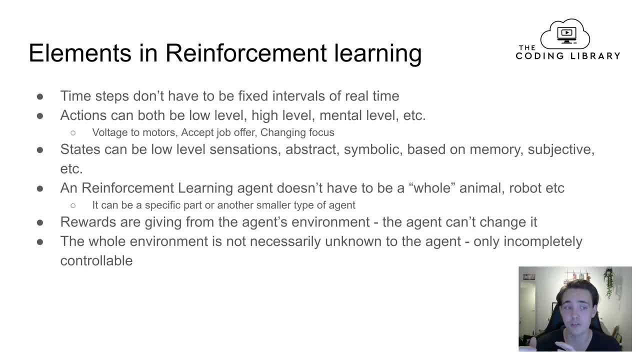 be like the real time or like a fixed interval of real time. it doesn't have to be like each time stick corresponds to, like each seconds that goes in real time, like at times that could be, um, when a new move has been made from the opponent in chess, then a new time step will. 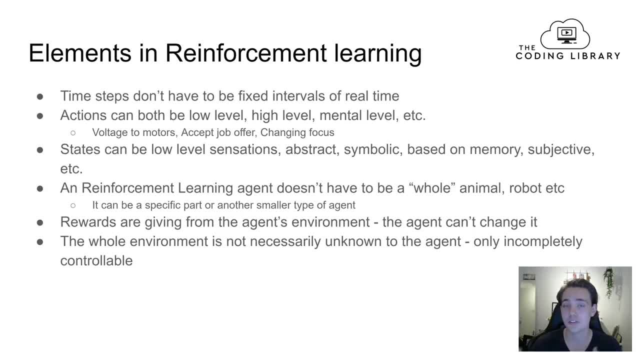 begin and then we will take an action in that time step. for some given state of that time step, where each time step could be like: every time it is your turn, then it is a new time step, and actions for an agent in reinforcement learning can both be like low level, high level or like 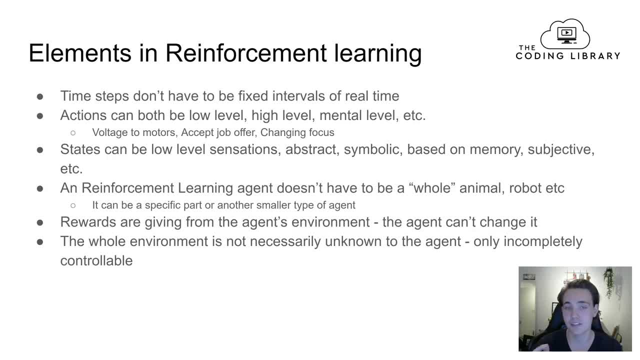 mental level. so we really like to define our actions ourselves. so we can like define actions of an agent to be like apply some voltage to motors which is really low level, or like some more high level applications where acts and an action could be accept a job offer if, if the agent 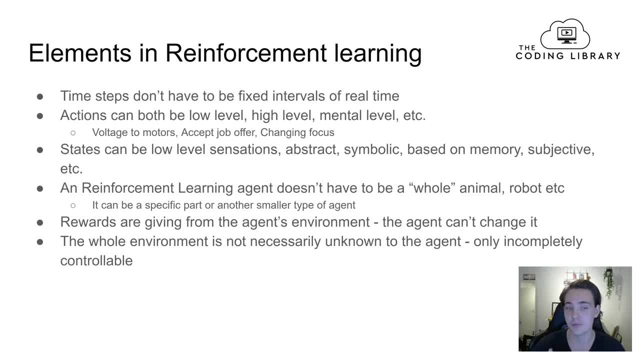 has learned that that's the properties or like characteristics of of a job. is is good and then we can have the robot taken an action of acceptance and job offer. and we can also like have um some mental level of actions. so if some is something like occurs like, then the agent can take an action. 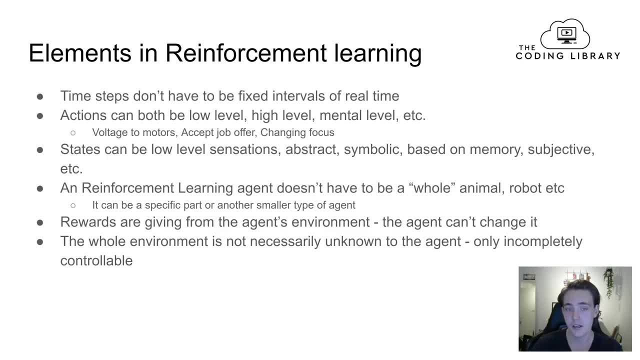 of like changing focus, for example, from one thing to another, um, for some given state, if that action is optimal and it gives the maximum reward, and the state states can also be low level presentations, abstractions, symbolic. it can be based on memory. so, for example, when we're talking about market, 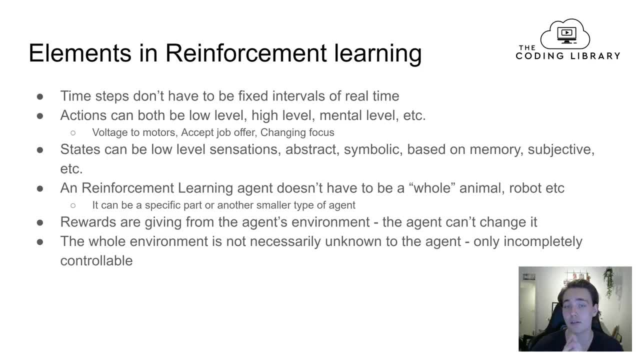 decision processes. um, we and we don't want to like depend on on the present and we have some like really important information from the person that we want to use, then we can actually like implement memory in our states and then we can have that, uh, that memory like that memory from. 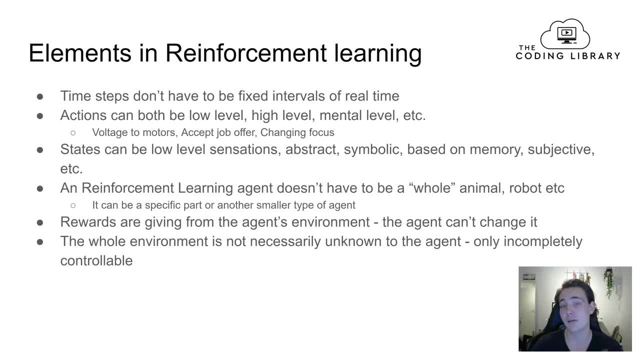 the previous states in inside of the given state right now and then we all then we actually like know something about the past in the given state now and we'll it will still have mock-up decision process. uh, property and it can also like the states can also be. 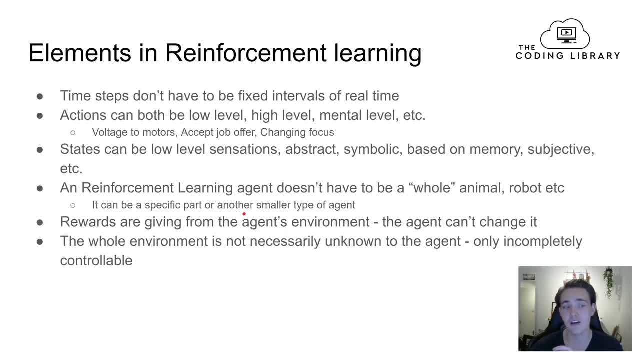 subjective and and etc. so we really like to find our states and actions and also like the time step ourselves when we're talking about reinforcement learning. and reinforcement learning agent doesn't have to be a whole animal or robot etc. like it can be a specific part or another, like smaller type of 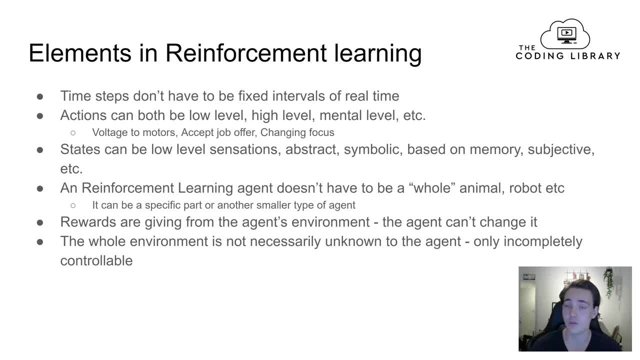 an agent like. it can be like, for example, if we're talking about a robot, it could be a robot arm, or like the head, or only like the, the legs, um, so it doesn't really have to be like a whole, a whole thing or agent, it can just be like: 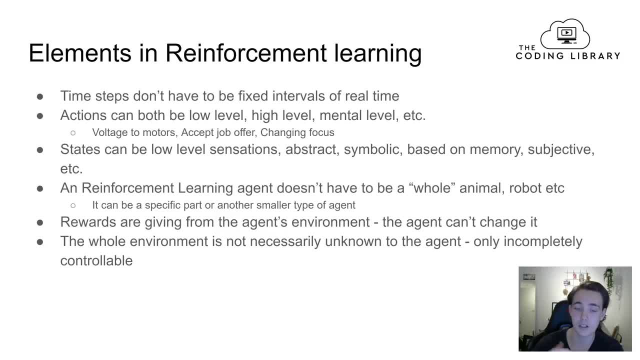 a specific part or some like computer, computer game or like a computer that tries to learn something. so again, we also different define our, our reinforcement learning agent by ourselves. so is it really up to yourself and what you define, your different kind of elements in reinforcement learning too, and it's also what makes reinforcement learning, uh, such a cool thing, a nice feature, and 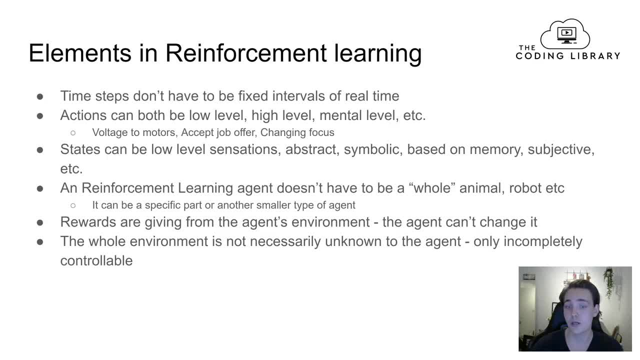 you can do, like almost everything you want to do with reinforcement learning, where you have an agent that you can place in in some environment and then it can try to interact with that environment and learn different kind of stuff to try to maximize the reward and get the maximum like like the maximum output. so rewards are also something we define ourselves. 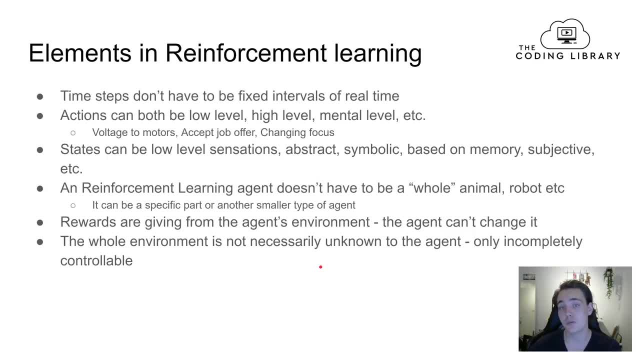 and it can be given from the agent's environment. but we should make sure that the agent can change the rewards and because we want to give the agent rewards on like how good it, how good it does and everything, so the agent shouldn't be able to change the rewards or like have anything with with. 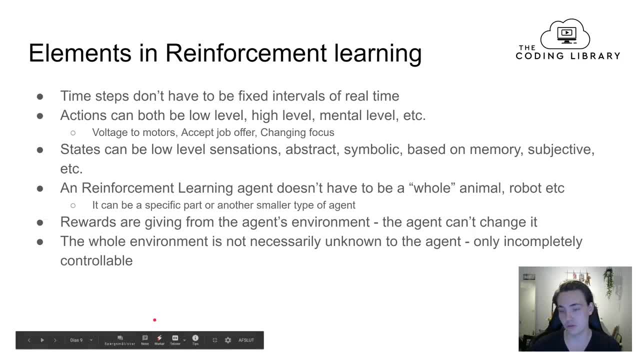 defining the rewards. so the whole environment is not necessarily unknown to the agent. like we could, we could feed information to the environment, to the agent, if we want to like learn it, have it learned faster or for some other different kind of purposes. so only incomplete, uh, controllable. 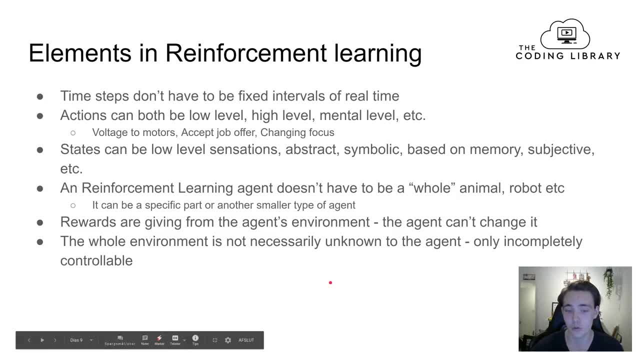 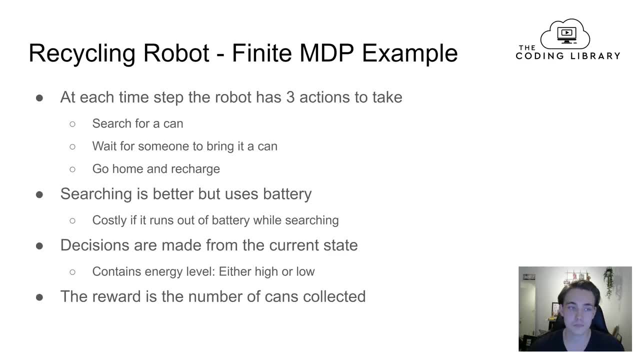 so the agent shouldn't be, shouldn't be able to control the environment. that is in because we should define the environment and then the the agent should only interact with the environment. so another example here we're going to have is a recycling robot, which is a also a finite mark of decision process example. so in this example here we have at each 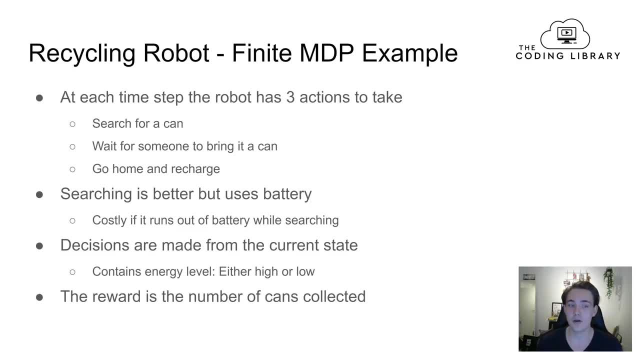 time slip. the robot has three actions to take, so we can either go out and search for a can, or you can wait for some someone to bring a can, or it could go home and recharge if it has used a lot of energy. so in this case, here on, our state will be um it will like also depend on the previous. 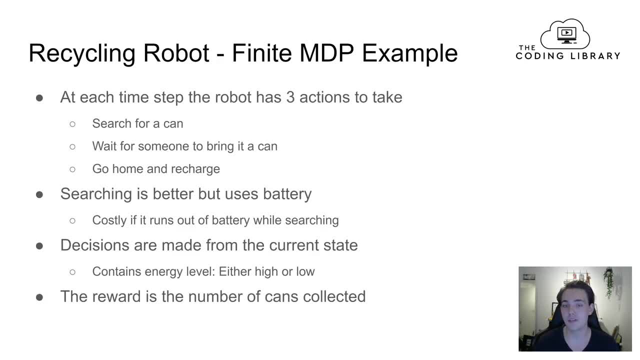 dates in when we're talking about like, because we're implementing memory in the given state now. so we will still have micro process because we just implement, like the previous states in the, in the present state now by having some like energy level um memory for our state now or and for our agent. 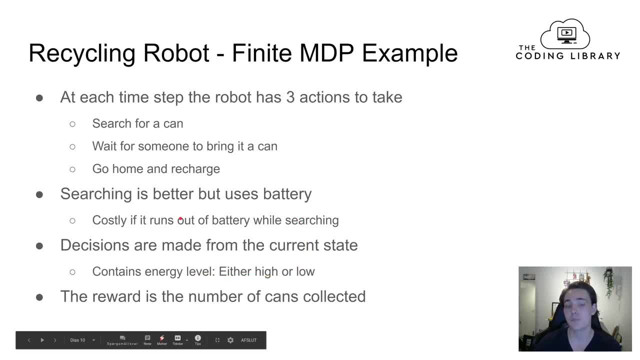 and then an example here: like searching is better, but you, it uses battery, so it is cough. it is really costly if it runs out of battery while out searching. um, if we have a robot arm or um that is trying to like pick up cans and or like is driving around trying to pick up cans and it runs out of. 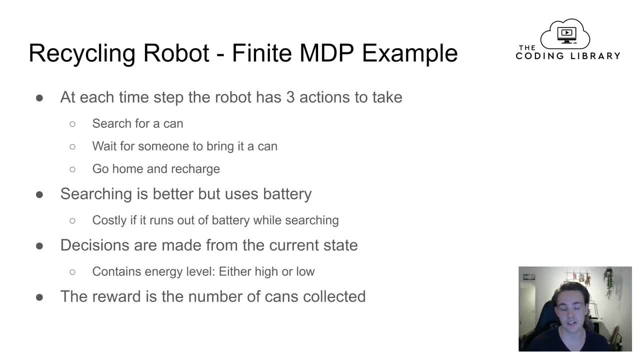 battery, then we will need to pick it up and and and put it back in the charger, which is, like, really costly and decisions are made from the current state, as I talked about, like it, but it contains the energy level, like it can either be high or low, so we still have this markup decision process. 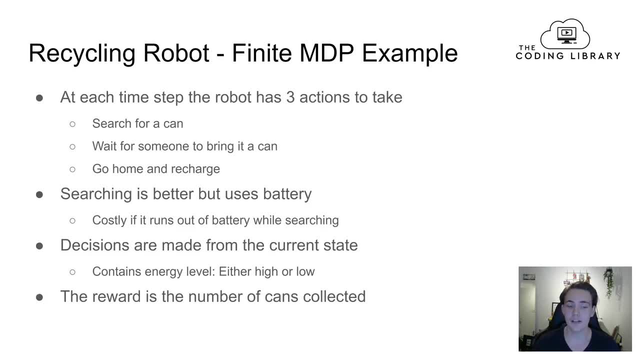 but we have just implemented some memory from the previous state as well. and then the reward is the number of cans collected for the robot, because we want to recycle as many cans as possible. the more, the more, the more reward our recycling robot gets. so in this case here we can set up like: 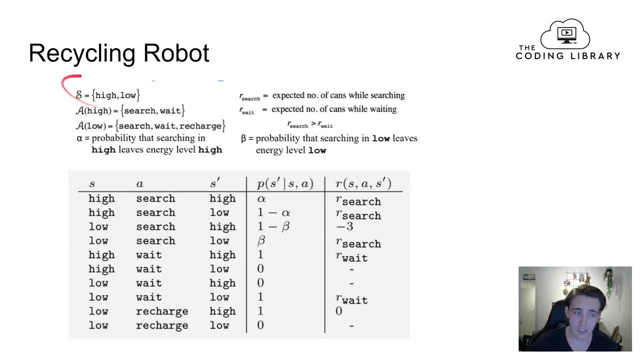 this scheme, or like this table here, where we have um a set of states here where it can either be high or low the energy level and we also have some, some, some actions which we can take if, if the energy level is high. so so we can take different kind of actions for a given state. so we can either like 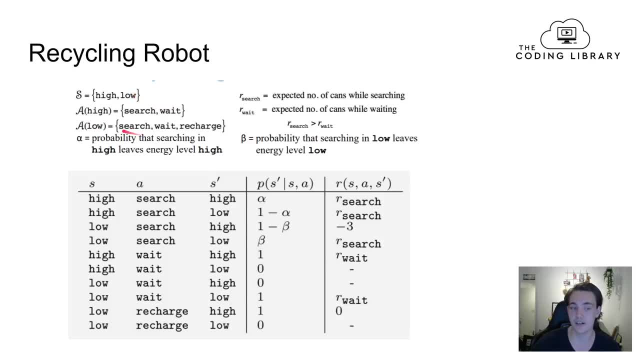 search and wait, or if our energy level is low, we can either search, wait or we can go home, and then we have this Alpha here, which is the probability that that's searching in high leaves energy level at high. so we we really want this um Alpha here to be to be high, because we need a high. 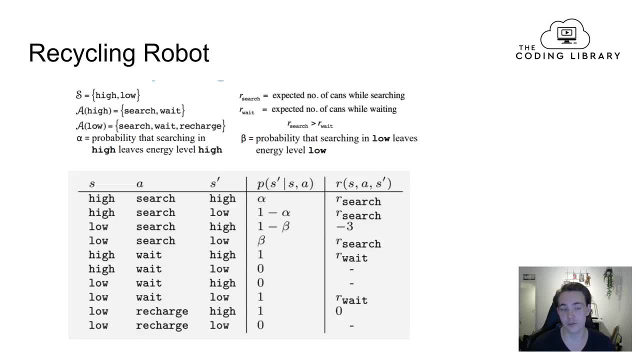 probability that we won't run out of energy when we're out searching. and then we have this better here, which is the probability that searching in low leaves the energy level at low, and then we can set up this table here for, like our, our different kind of actions for a given state, and then we can 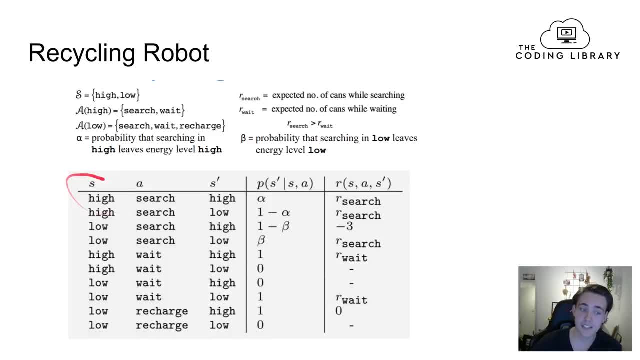 just going to get a go over, like some of the examples here, where if we're in the state here and we have high energy level and we're searching like, then the probability here of the next date is like the probability of that we're still at the high level energy level in the next date is is. 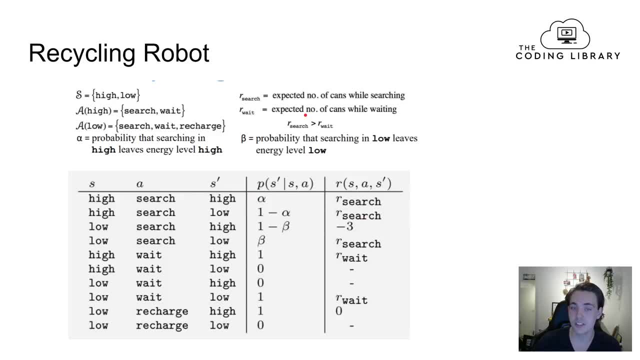 still high. it is Alpha here and then the r search. here is the expected number of cans while searching, because the reward here was the total like. we want to maximize the amount of cans that we're returning. so keep doing this here for the given sets or like the given states and actions that we can take. so 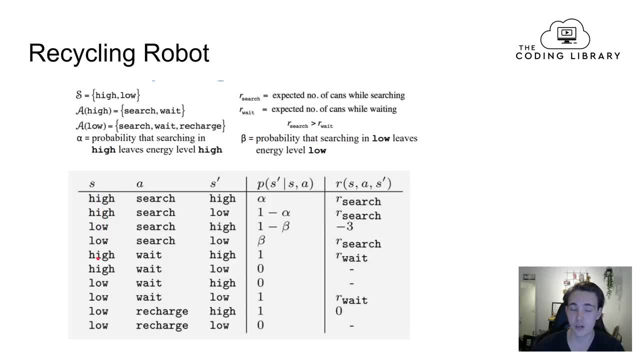 we have these different kind of states, like states. here we can be in for a robot, robot's energy level, and then we can either search, wait and recharge and then the probability and that the next date that we we can go to, the next date when we give, when we give it a state and an action, and then 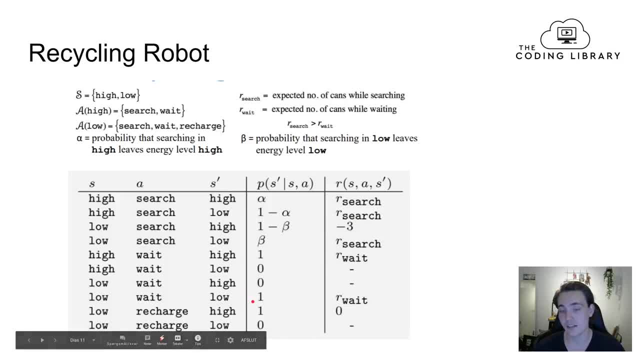 we can set up like the probabilities here um for the energy level, and also we can set up like the here for our searching and waiting and the different kind of like states and actions, and also it also depends on the next dates we can take. so then we can set up this scheme here like table. 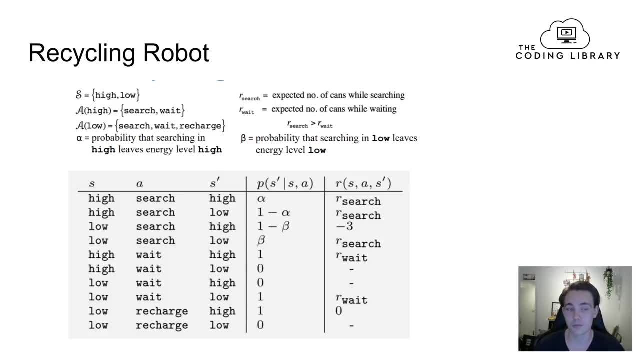 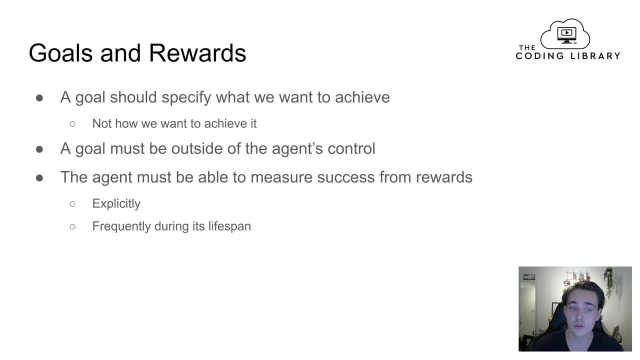 here, and then we can have our our robot learning with reinforcement learning. so the next thing we're going to talk about here is goals and rewards in reinforcement learning, where a goal should specify what we want to achieve and not how we want to achieve it, so we don't really care, like how. 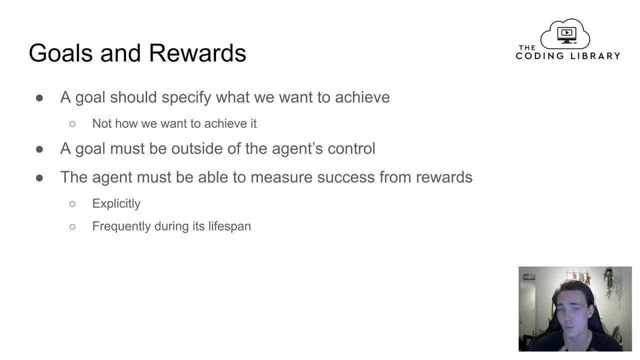 um, how we're going to achieve it. we just like want to specify what we want to achieve and then our robot will try to to get to that point. and a goal must be outside of the agent's control, so the agent shouldn't be able to change the goal. we 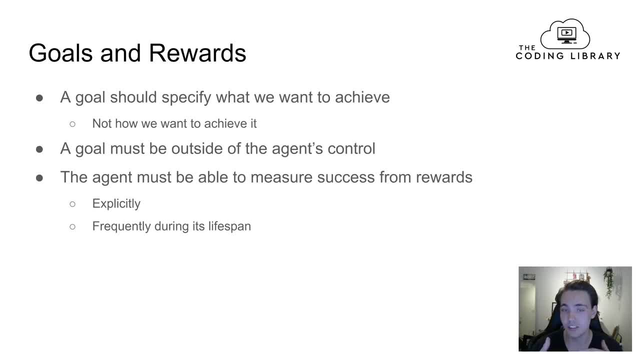 want to set the goal for the agent, and then that agent should try to reach the goal, not try to modify it or control it, and and in some way. and then the agent must be able to measure this success from the rewards. it can either be explicitly or frequently during its lifespan. so the agent must 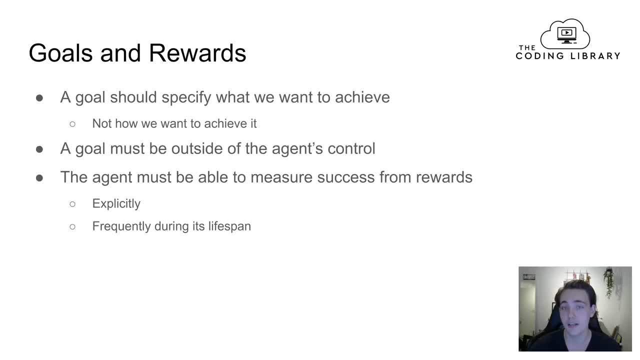 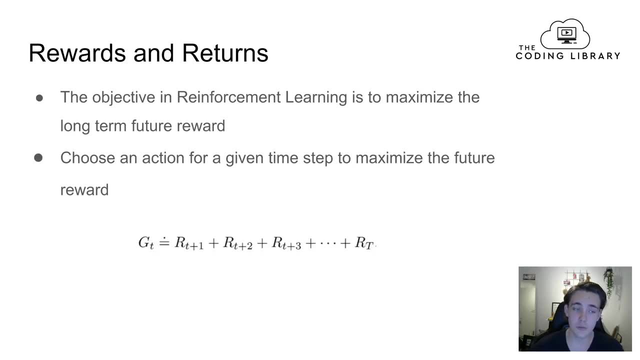 be like how good it, how good it performs and how good is learning by getting these rewards and trying to maximize- uh, try to maximize the reward it gets. and then we have rewards and returns where, like, the objective in reinforcement learning, as I've already like said many times- is to maximize. 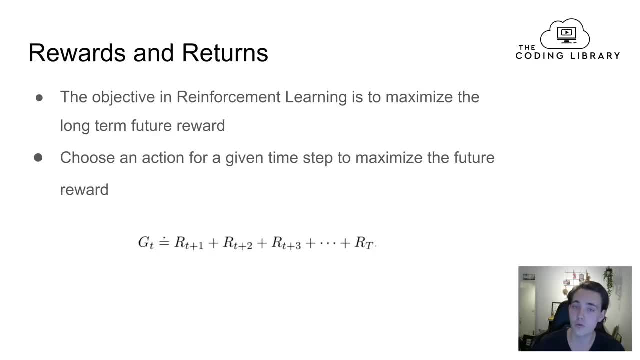 the long-term future reward. so we want to have our robot trying to reach, to go to the goal and return the maximum number of reward, and then we choose an action for a given time step to maximize that future reward. so in this case, here we just have a sequence of. 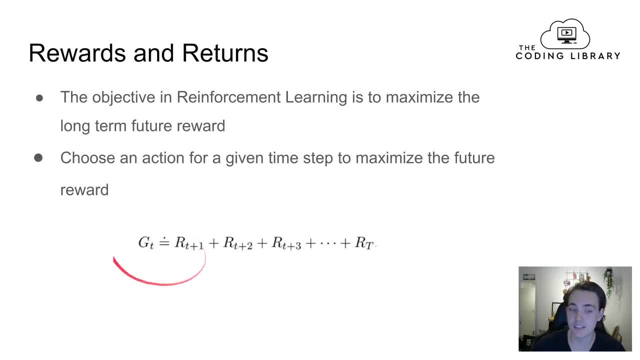 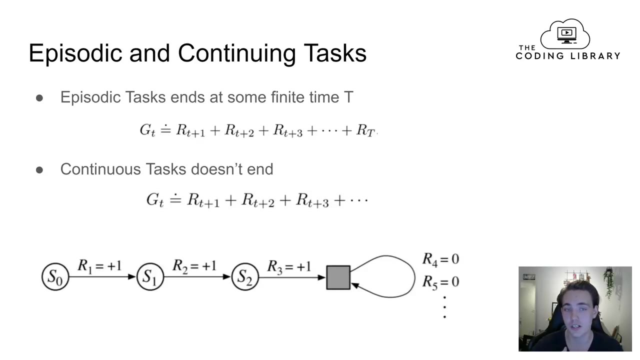 rewards and then we try to estimate or, like this, maximize the reward. so then we just like: add all the rewards for each time step that we're going in and then we get that maximum reward. but we can also like, when we're talking about episodic, we can have either of episodic and continuing tasks. 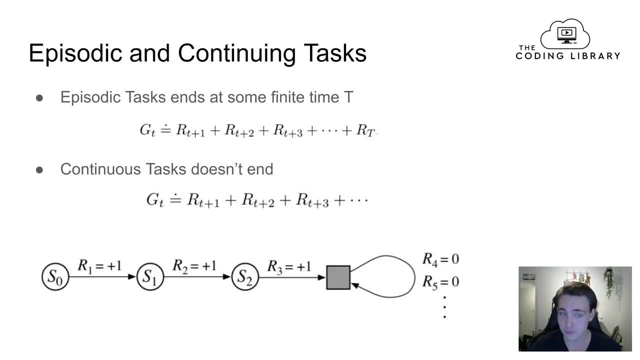 in reinforcement learning. so when we have an exotic task, it ends at some finite time T. so we have some tasks and we have some episodes that it's going over, like, for example, when we saw the example with open AI where we had these agents playing hide and seek. then an episode and ends if 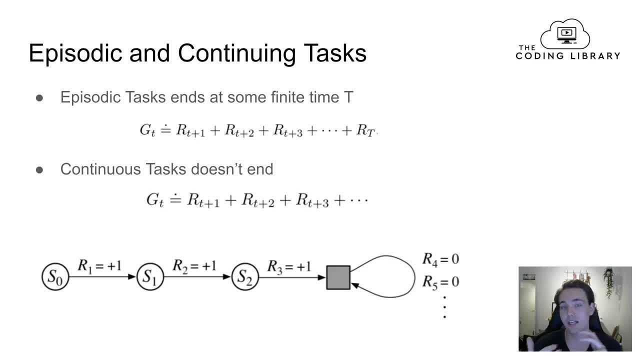 the agents get, uh, get are found, or it also ends if it can't be found as well, and then we can like calculate the rewards by just adding them all together and then we can see, like how good our, our agent has performed. but we can only have this continuing task that doesn't end and we don't have. 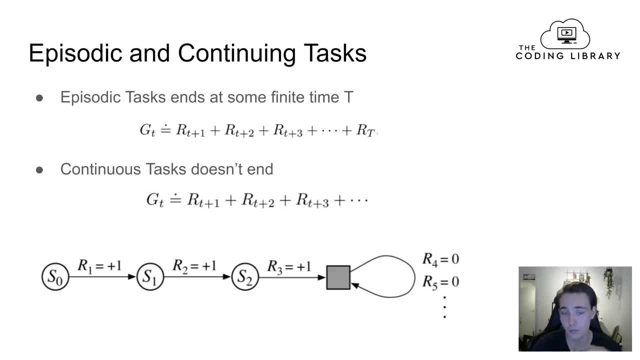 time. so then it's like a bit harder to calculate the reward because we don't know, like how, for how long it's going to, how long it's going to keep on going, because it's just a continuous task. but we can actually like make our um, our episodic task continue as well if we just have this loop here. 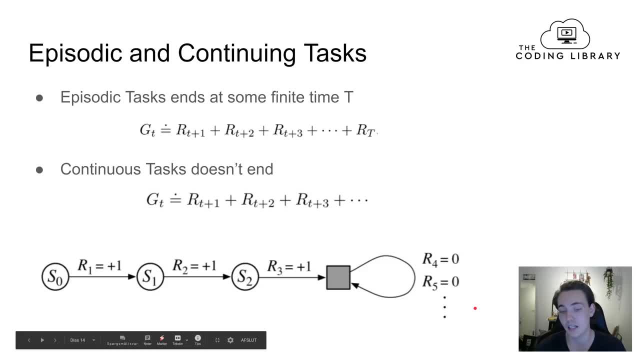 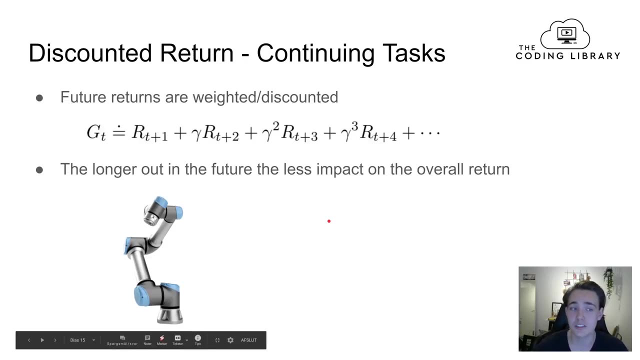 we just goes and goes back and then the reward will just be like at the end of the sequence and we don't want to like terminate our, our episodic task or terminate our task. then we can just have this loop going back and then the reward will be zero. so when we have this continuing task here, we also need to have this discounted return. 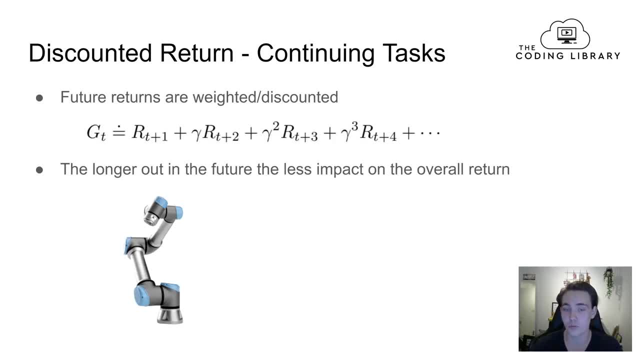 because then we can just add up all the rewards, because we don't know all the rewards, because we don't have a finite time where it um, where our episode terminates, so we can have these future rewards, that that are weighted or like discounted. so we're talking about the discounted rewards when 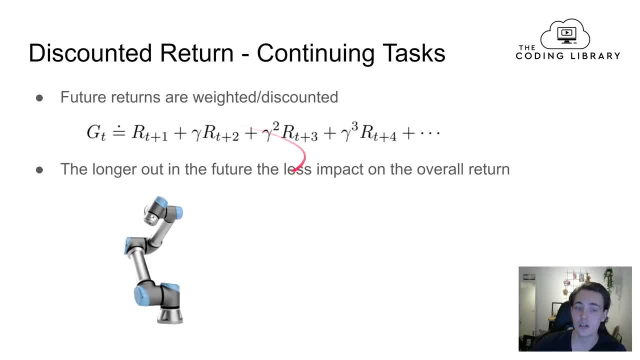 we have continuing tasks, so and then we discount our um, our return here, with this gamma factor here. so the longer out in the future our, our, our rewards are like, the less impact they have. so we can see that we don't scale the reward at the next time step here by anything. and then the longer we come out or like, the longer we come. 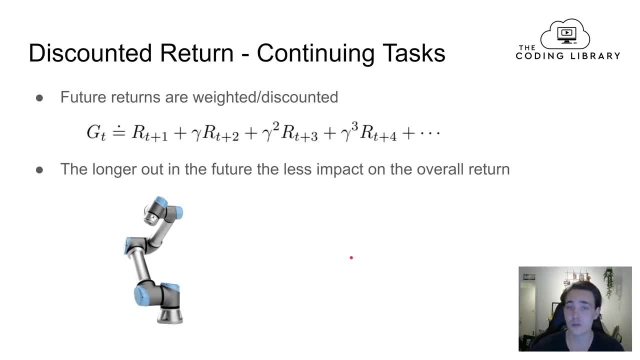 out and in time step like the less impact the reward has. so so the robot tried to take an action. um, depending on the next date and a couple of next days and not the reward, it gets like a long way out in the future. so the longer out in the future it's less impact on the overall return and 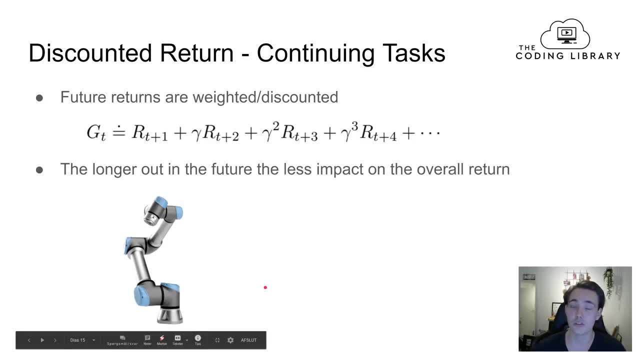 so an example of continuing task could be a robot arm that that is just doing some picking or like at some manufacturing, where it's just like picks items and places at another, like another place, or an appell um, and then it will be a continuing task and we should take the action. that is that 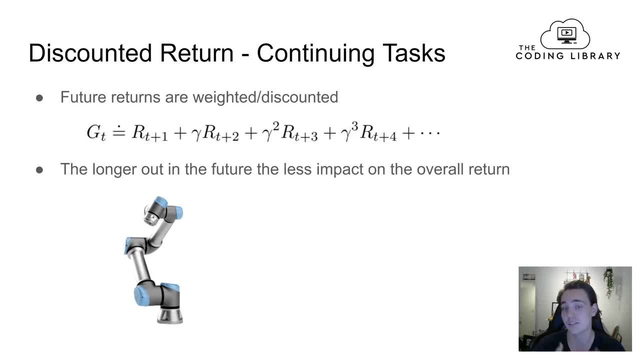 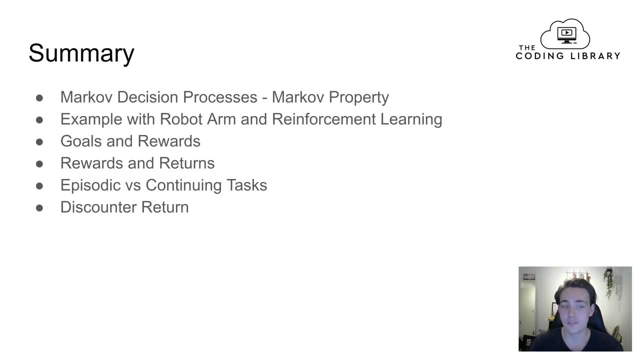 is best for the next time step and not, um, not that it gives a better reward, like in two minutes, and stuff like that. so just to summarize what we've been over in this video view, we have talked about mark of decision process and is, and we talk about what the mark of property was and how we can, how we can see if our process 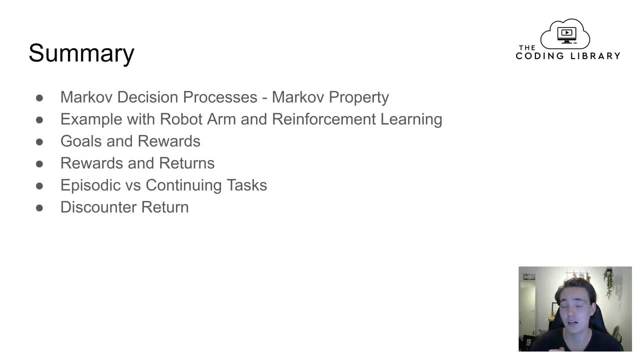 has this markup property by not depending on the previous states and only by the state we're in now, and then we could implement some memory from the previous states into our, into our agent, and it will still have this markup decision process. we also went over an example with a robot arm and 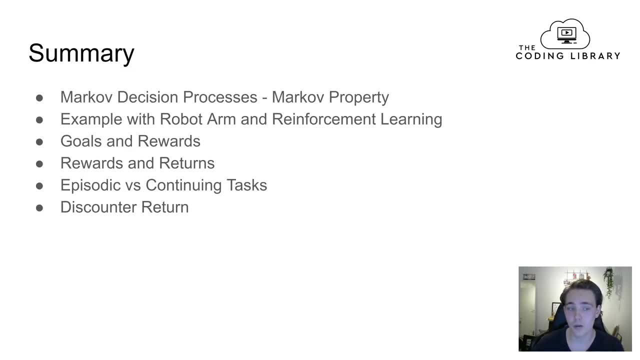 reinforcement learning with this recycling robot, and we talked about the goals and rewards and the rewards and returns, where a robot has a goal that is that it wants to reach, and then it tries to maximize the rewards all the time to reach that goal most optimal and then in the end we're talking. 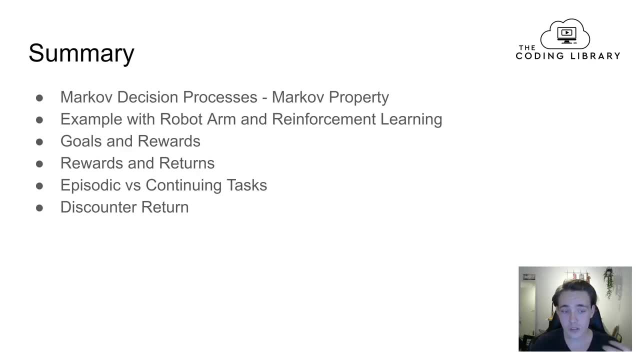 about the episodic and continuing task where where, if we had a continuing task, we needed to have this discounted return. so the longer we come out in the future like, the less impact the returns has, because when we have this continuing task, we don't have a defined like a finite time step where our 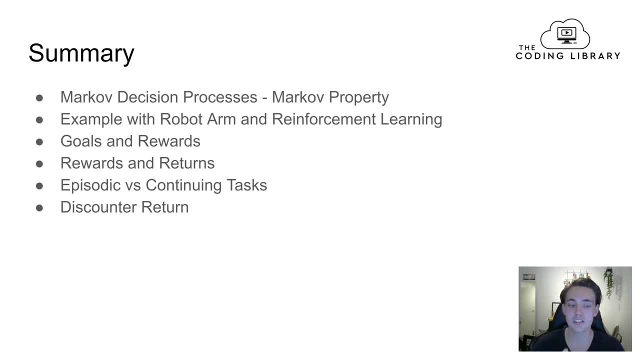 every epic episode ends, so we need this discounted return. so our action is based on the rewards for the next couple of time, steps, or like the next couple of rewards, and not that much out in the future. so thank you, guys, for watching this video and remember to hit the subscribe button. 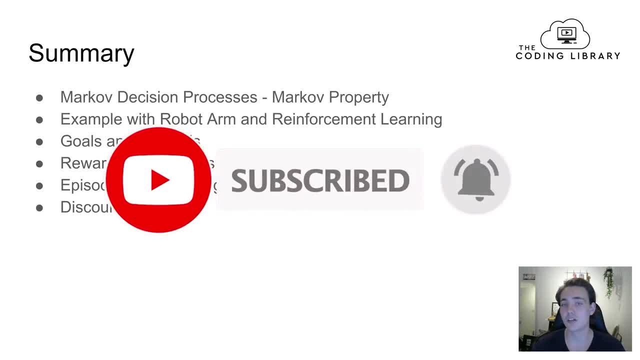 and bell notification on the video and also like this video if you like the content and you want more of it in the future. so i'm currently also doing a computer vision tutorial in opencv in c++ and an algorithm data structure tutorial in c++ as well. so if you're interested in one of those, 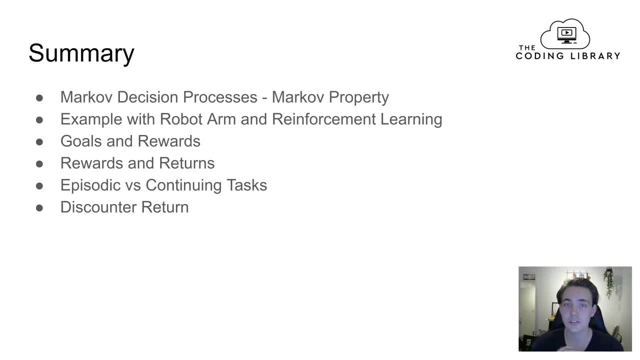 i'll link to one of them up here, or else on to seeing the next video. guys, bye for now.